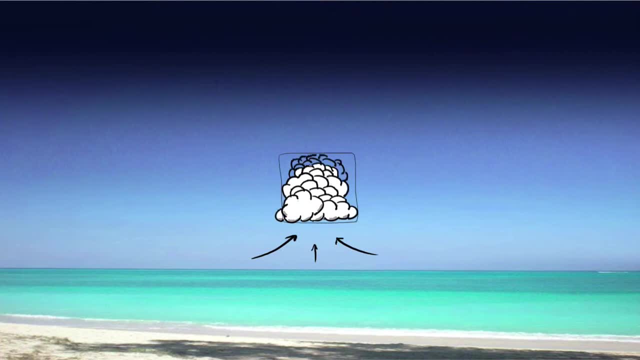 This helps to warm the cloud, which makes it climb higher. But the higher the cloud rises, the more it expands And the cooler it gets, More moisture condenses, which warms it back up, making it climb higher, Up and upward. it billows in a reinforcing feedback loop of expansion. 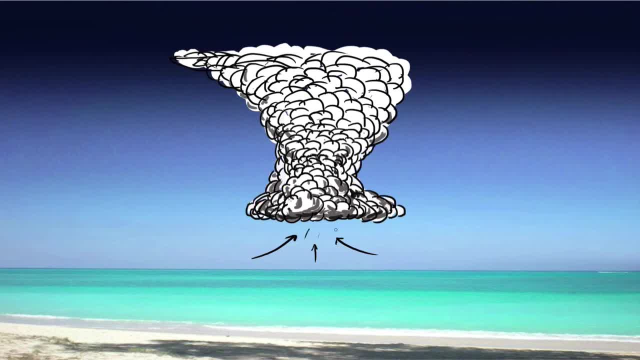 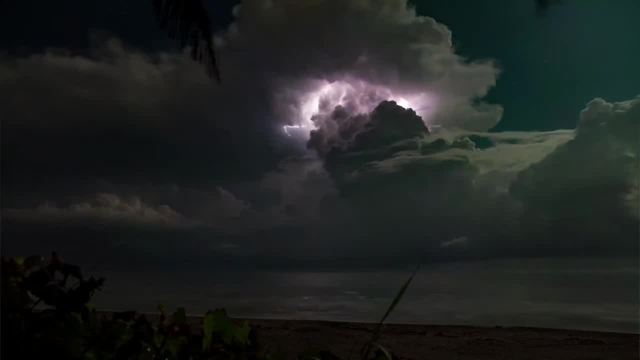 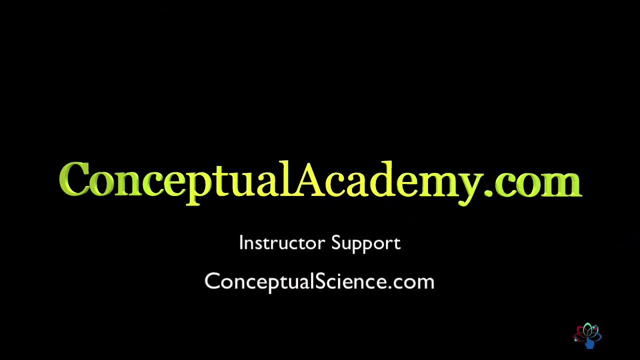 followed by cooling, followed by water condensation. Eventually, a thundercloud is formed. Good energy, How Excelent 빠� you big lose. how big you year Obama. last time, strong downloaded your new Cloud Nutrition very easy, a really simple way. to transform. 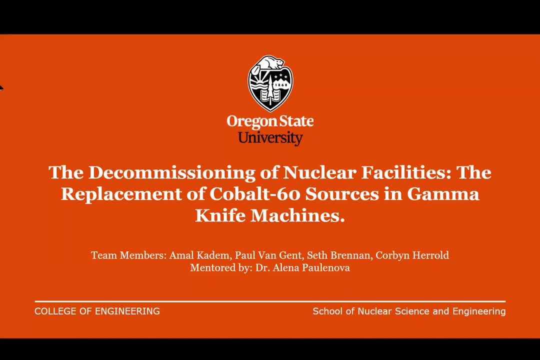 And welcome to our presentation on the decommissioning of nuclear facilities, the replacement of cobalt 60 sources and gamma knife machines. My name is Paul van Ghent and my teammates are Amal Kadam, Seth Brannon and Corbin Herold. We are mentored by Dr Alina Polanova. Next slide, please. 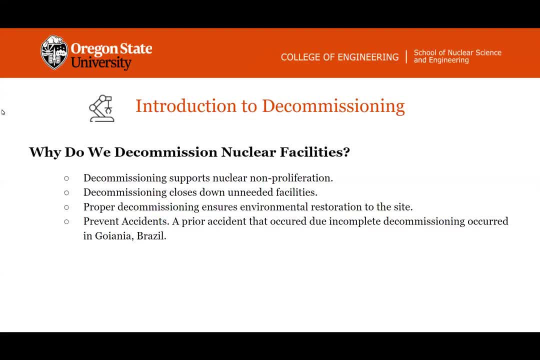 Before we explore the decommissioning, it is important to understand why decommissioning is done. By decommissioning we can ensure that nuclear non-proliferation goals are achieved by continuing to secure nuclear sources. Decommissioning also ensures that work is done to restore the environment after a facility is closed down. 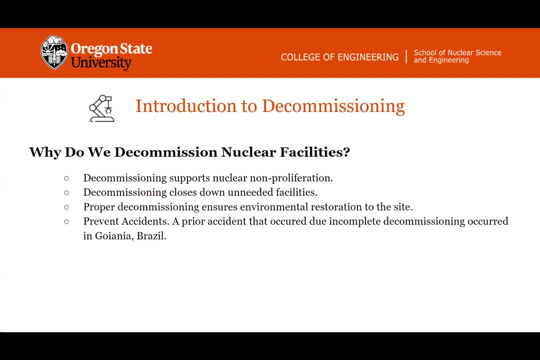 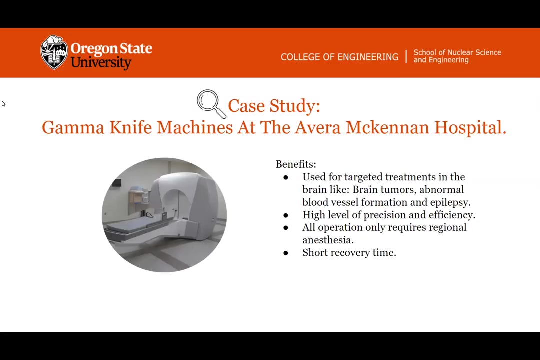 Decommissioning's importance is shown by prior accidents that have occurred, from immigrants or other accidents. Decommissioning also ensures that work is done to restore the environment after a facility is closed down. Decommissioning also ensures that work is done to restore the environment after a facility is closed down. 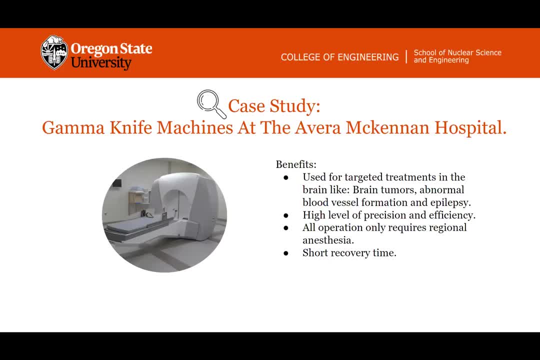